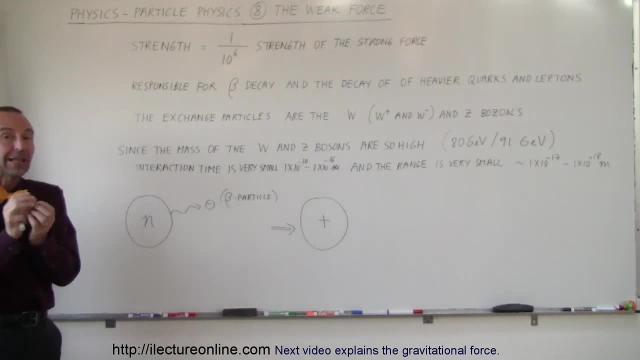 but it acts over a very small range, much smaller even than the nuclear strong force, And it is responsible, or at least it's theit gives us the interaction that provides the beta decay and that provides the decay of heavier quarks, For example. the beta decay is the ejection of 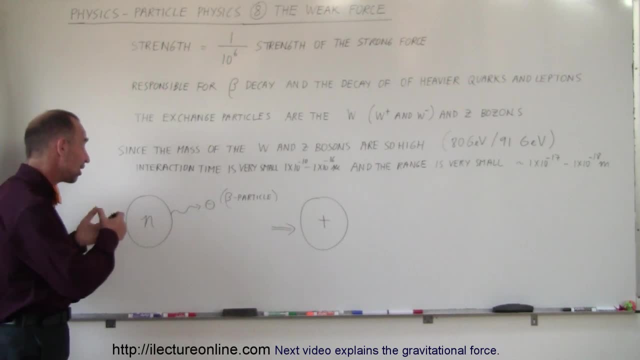 an electron from the nucleus of an atom and typically that's the ejection of an electron from a neutron in the nucleus of an atom. So when a neutron ejects an electron, a beta particle, the reason why we call an electron a beta particle because it's ejected from a nucleus. or ejected from a neutron. it turned out to be more favorable for theta, uha, grubTA, or an electron which bakes the our filters, which can produce more diagonally and more Quarkoholically. When a neutron ejects an electron, they always respond to the data that makes them. 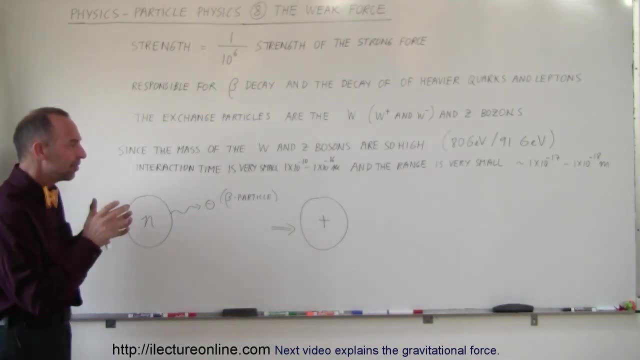 more Pearson. you know what I mean. something like that. So without these particles, weiere not only turns a neutron into a proton. So by doing that, since the makeup of a neutron and the makeup of a proton is determined by the types of quarks that are in there, that must mean that when it 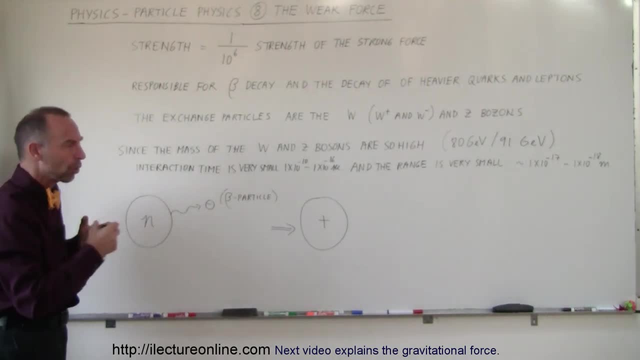 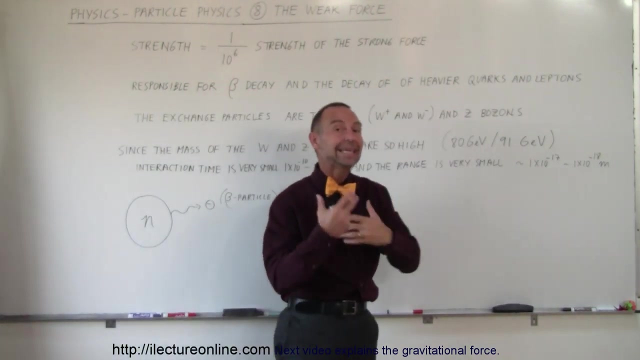 ejects an electron, it must change one quark into a different quark, And so what we know is that the interaction that's caused by the nuclear weak force causes this decay of particles and makes it change from one to another, Especially the heavier quarks. there is a set of heavier quarks. they 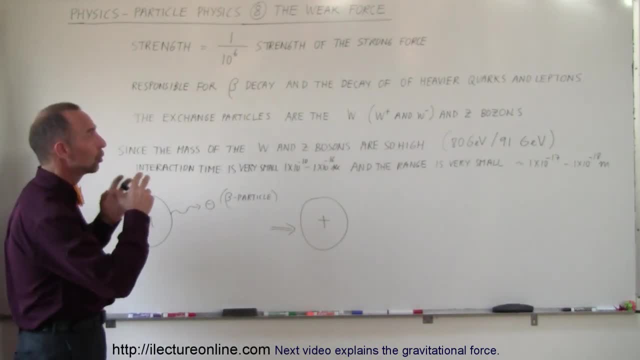 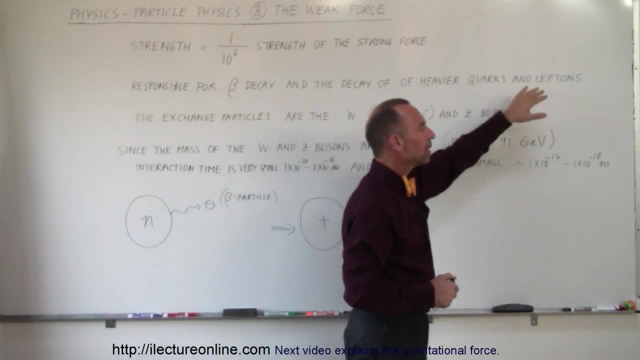 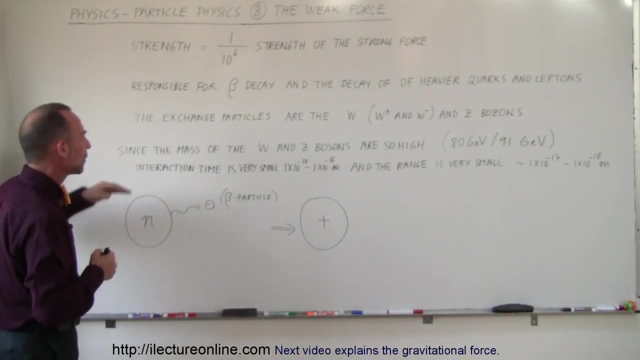 decay into different quarks by this nuclear weak force interaction. Also, the decay of leptons can also occur due to the interaction of the weak force. Now, what is that? How does that work? Well, actually we discovered that there are exchange particles. this was back in the 1980s, so it wasn't 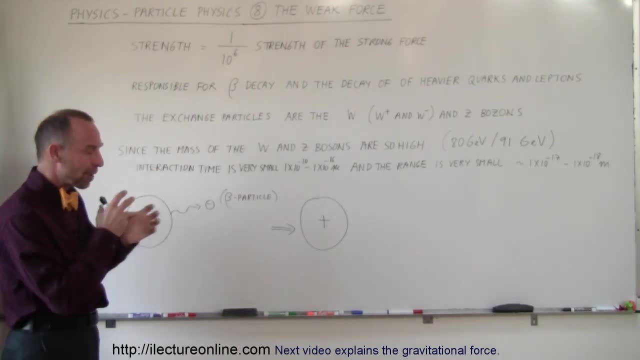 that long ago that we discovered that the interacting particles that create, or that at least are the messengers of the nuclear weak force are the interlocking particles, And so what we know is that the interlocking particles, the message carrier of the weak force, are called. 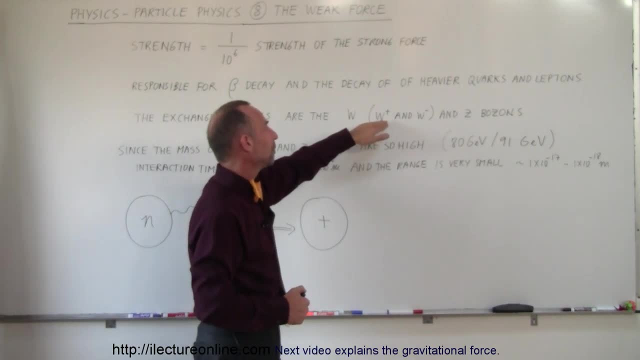 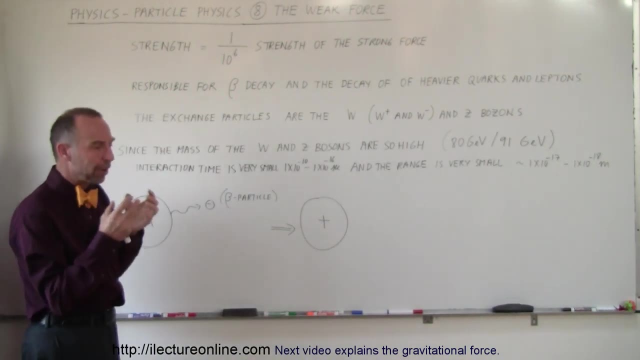 the W and Z bosons. Now on the W bosons we have a positive and negative charge type, and then we also have the Z bosons. Now the bosons are particles that have no structure to them. They're like point objects. It's kind of like an electron is a point object. There's no visible structure to. 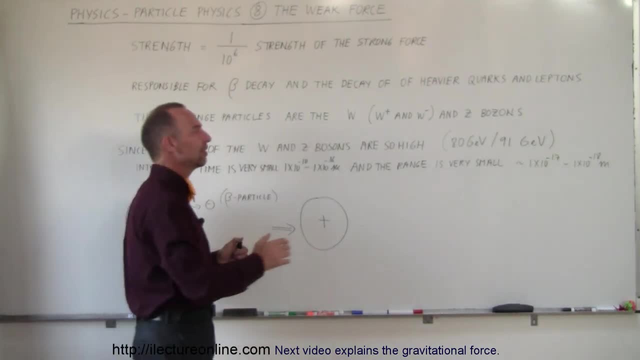 the bosons, But yet they're extremely massive in size. The W bosons are 80 giga electron volts and the Z bosons are 80 giga electron volts And the Z bosons are 80 giga electron volts And the Z bosons are 80 giga electron volts And the W bosons are 80 giga electron volts And the Z bosons are 90 giga electron volts. And the Z bosons are 90 giga electron volts And the Z bosons are 91 giga. 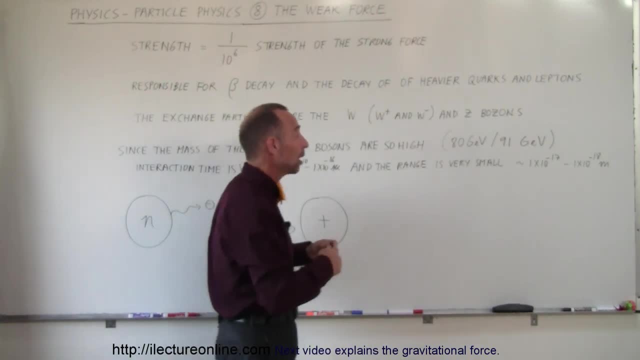 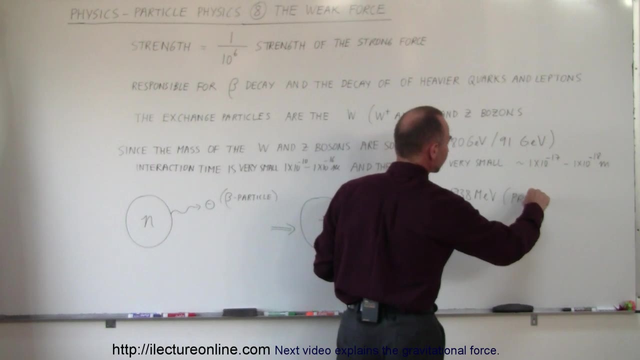 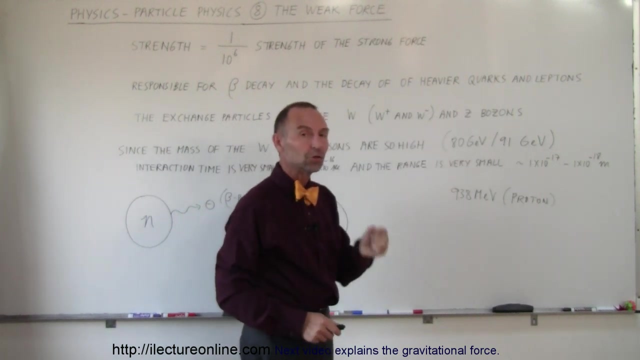 electron volts in mass. Now to compare that to the proton, a proton is about 938 mega electron volts. for a proton or a neutron, A neutron is 939 mega electron volts, But you can see that it's roughly 100 to 1.. So the mass of a boson, which is an interchanged particle of the weak force, is 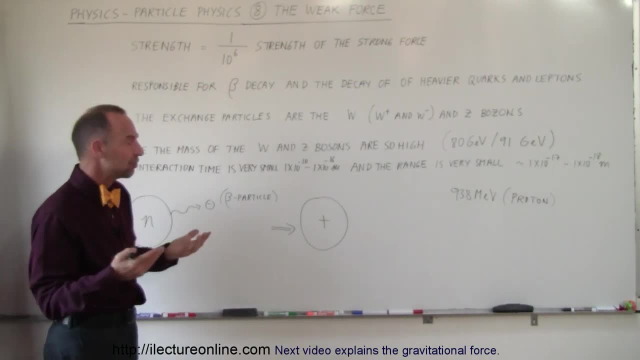 100 times as massive as a proton and neutron, which is kind of interesting. How does a particle that is 100 times the mass of a neutron be the cause of the ejection of an electron, a beta particle, and causes one quark, which is very tiny in comparison to the mass of a neutron, to change to a different? 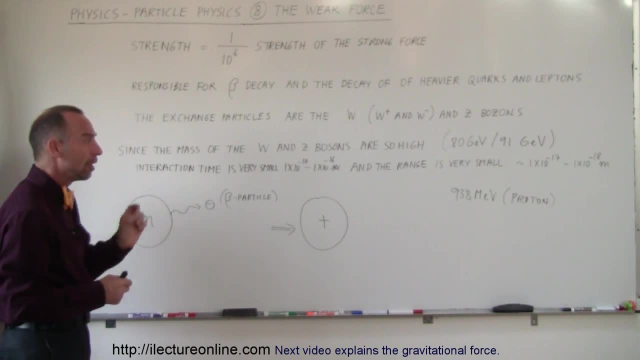 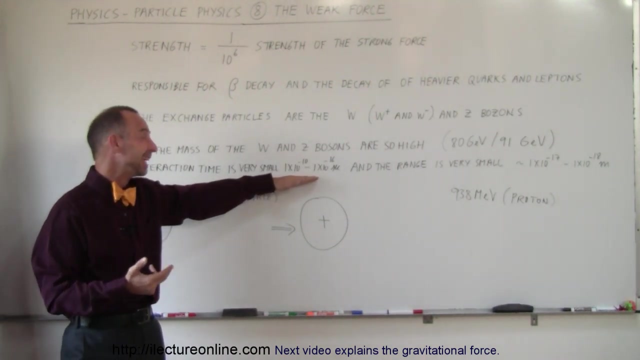 quark, Very, very strange how that works, But the answer to that is that the existence of a Z boson or W boson is very, very short. It only exists for a very tiny amount of time. For example, the interaction time is extremely small, anywhere from 1 to the minus 10,. 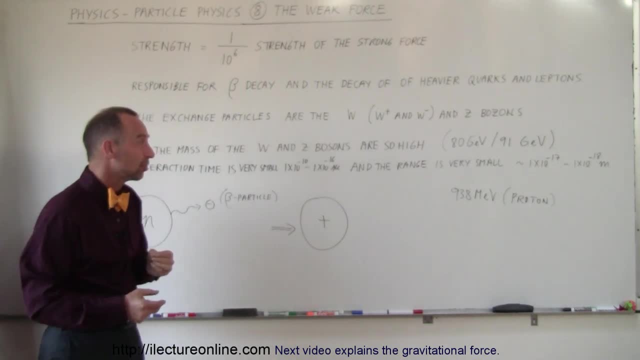 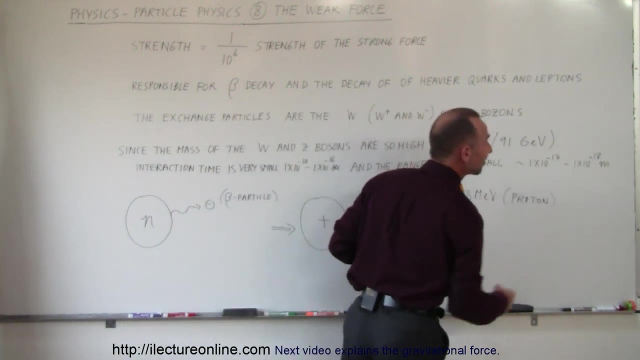 10 to the minus 10 to 10 to the minus 16 seconds. So therefore also the range is very small. Notice that the range is somewhere in the order of 10 to the minus 17 to 10 to the minus 18 meters. 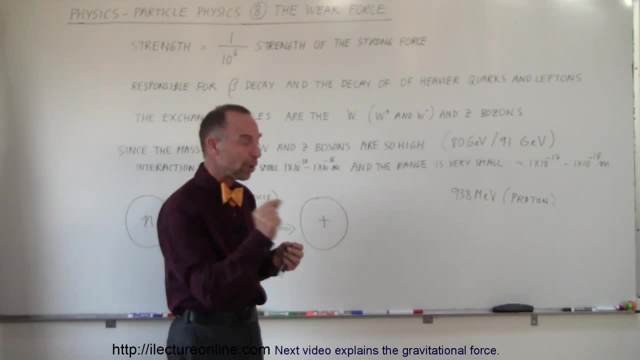 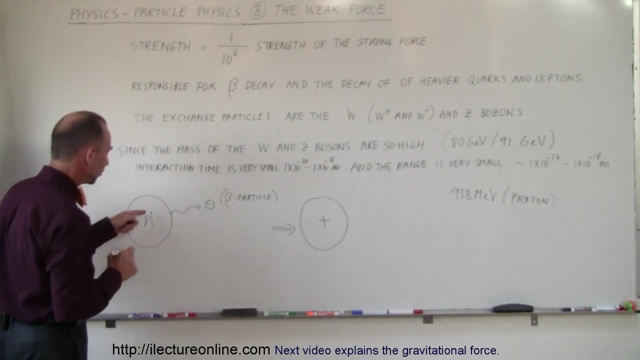 which means it's somewhere in the order of 1,100 to 1,1000 the diameter of a neutron. So imagine that the range is a very tiny little range, somewhere like that, for a very short period of time. And what happens is, for that very short period of time, a boson is created. 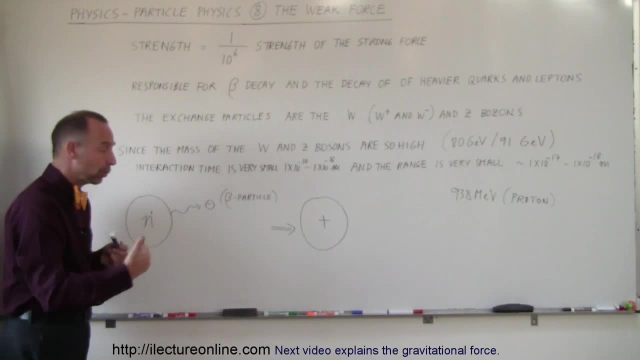 that causes the split up or the change of one quark to another, and that causes the ejection of a charge in the form of an electron in order to make that change happen. And so the nuclear weak force- we call it a nuclear weak force- is such a force that the reason for that force is the decay from one. 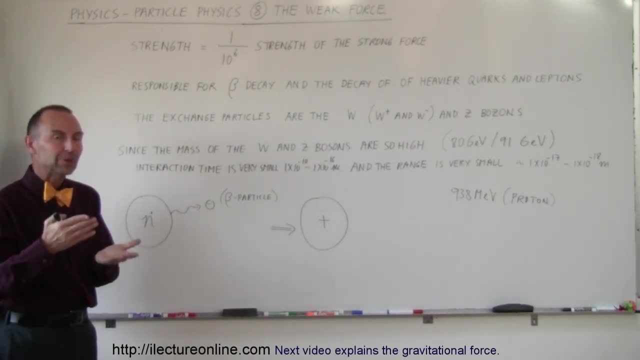 particle to another. Now we've discovered hundreds of particles already, with the vast majority of them being very unstable. So if you ask for a very small fraction of a second, then typically they interact to this weak force and cause the ejection of neutrinos and electrons and photons and so forth to carry off the energy.